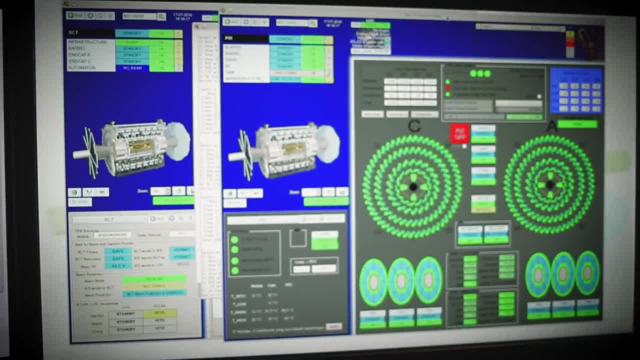 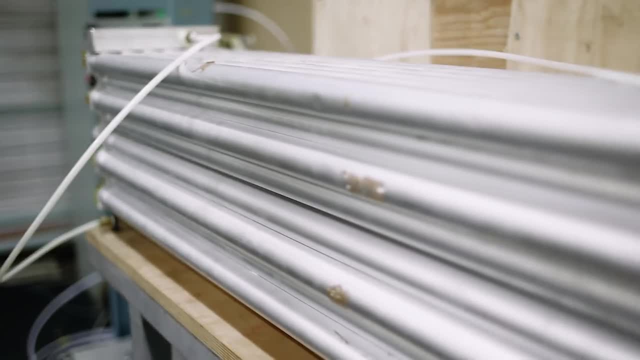 need to man the experiment. We need to have shifters monitoring the detectors, the data that we're taking, and make sure that everything looks like it's expected and also make sure that nothing's going wrong. They're called MDTs. They're a bunch of drift tubes. They're actually like what's in the muon. 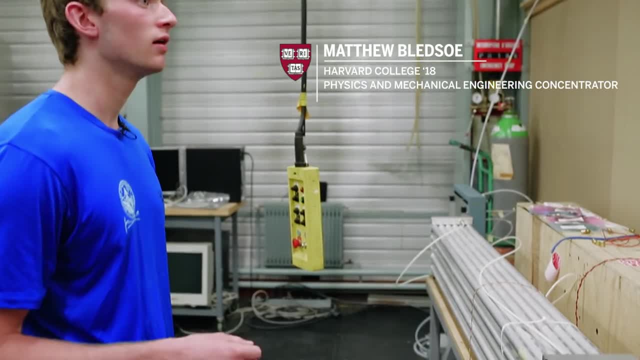 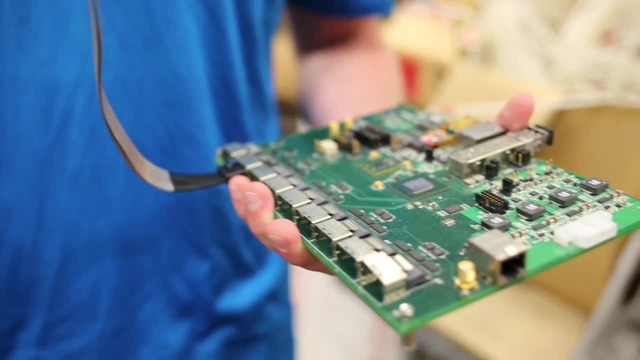 detector of ATLAS right now. We're replacing these with something that's like much more sensitive, Like I think there's 300,000 tubes on the detector right now and the replacement that we're making is going to have like 2.5 million channels, So it's going to be like a lot more. 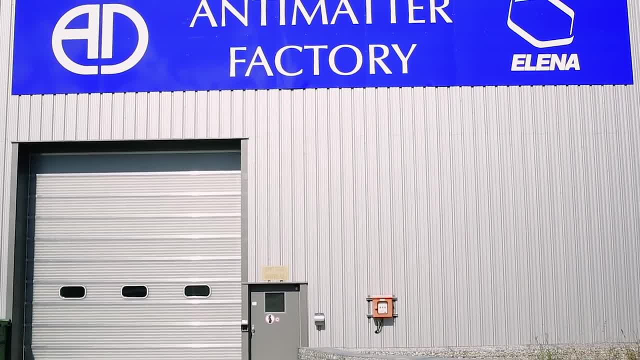 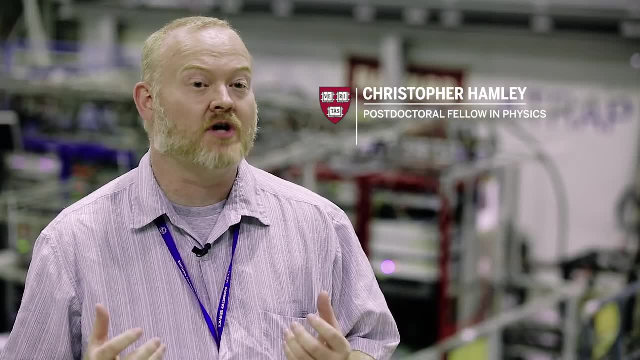 sensitive and read out data faster. So the building we're here at CERN is the anti-proton decelerator facility. CERN sends protons from the proton synchrotron to us. They hit a target and produce proton-anti-proton pairs. 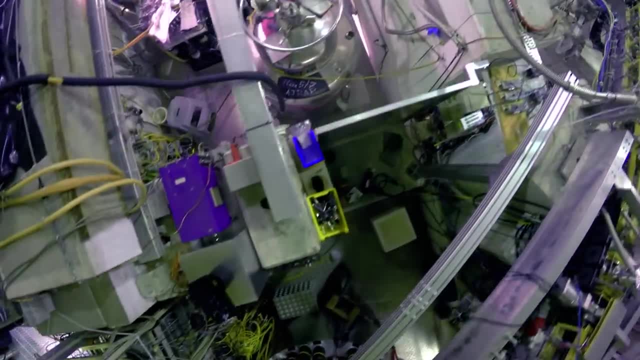 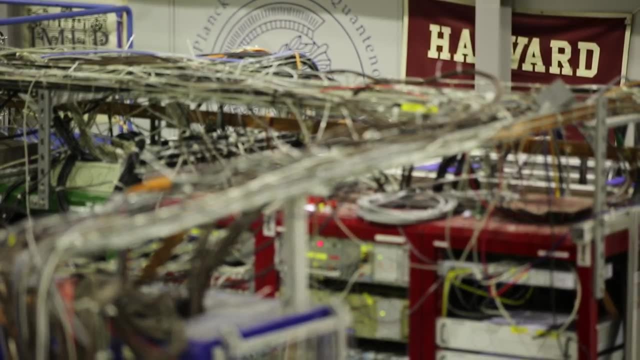 which are then captured in the deceleration ring And they run them around the ring, decelerate them, cool them so they can supply anti-protons to the experiments here, And this is the only source in the world for anti-protons like this. I think we know a lot about antimatter. 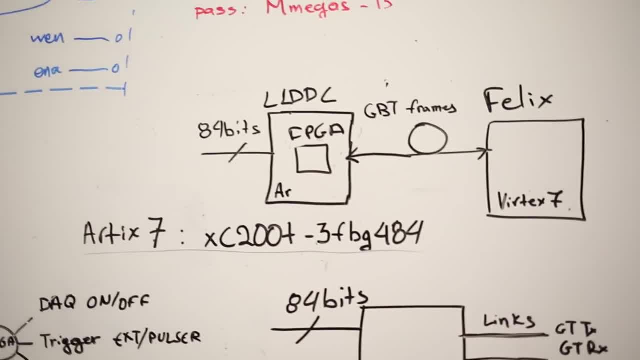 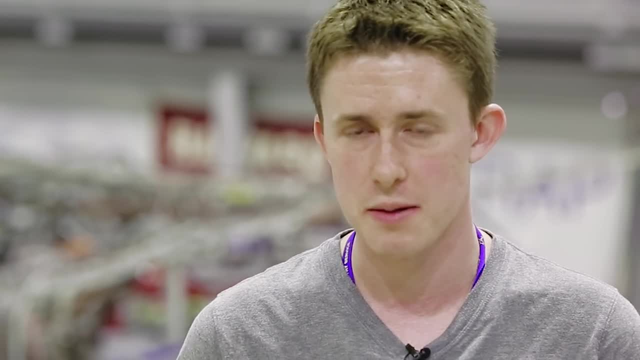 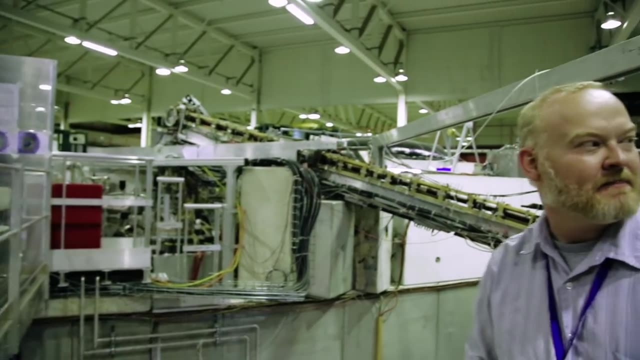 The question is whether there's actually a difference between the two. You look at the universe and of course you see matter And not so much antimatter. But when you look at the fundamental equations, they seem symmetric in matter and antimatter. So the question is: how do you get this universe full of matter? 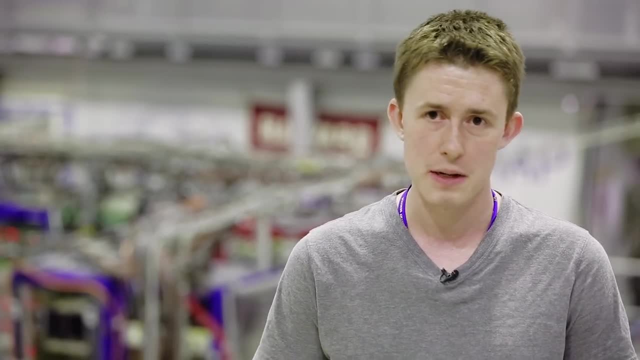 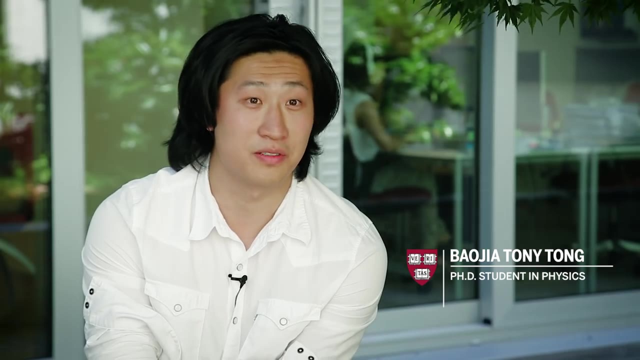 from equations that treat them more or less the same. It's always helpful to answer the question of why- why skies are blue and why the universe is so big- all this basic stuff. I'm always curious about these questions and the solution. 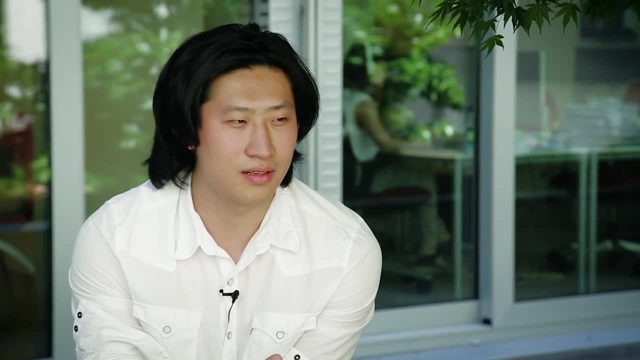 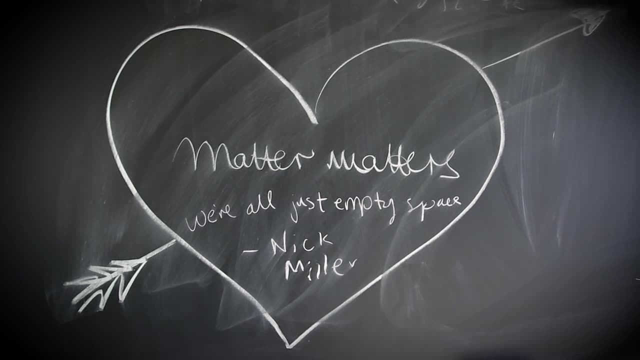 is always so beautiful Of answering those questions, truly amazing. and it's like the physics is all we know, right? It's like everything: The more physics we know, the better we know where we are, where we are going and all these questions. 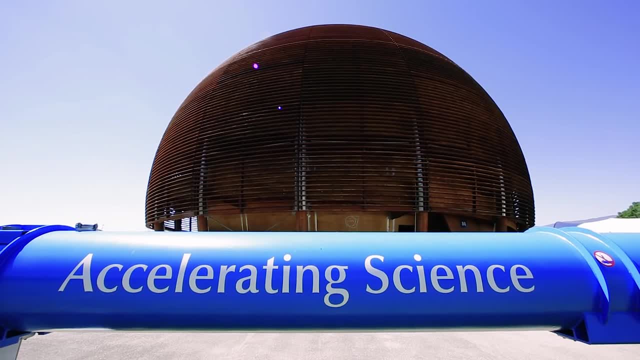 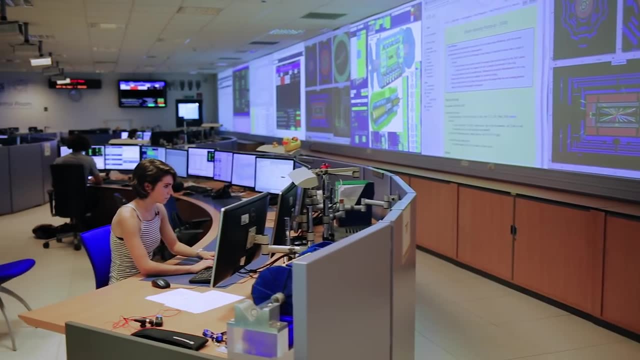 As a scientist, you like asking nature questions and seeing what the answer is. Because we have thousands of people working on a single experiment, you know that we're asking some of the most difficult questions in the universe. So that's what I really like about CERN is. 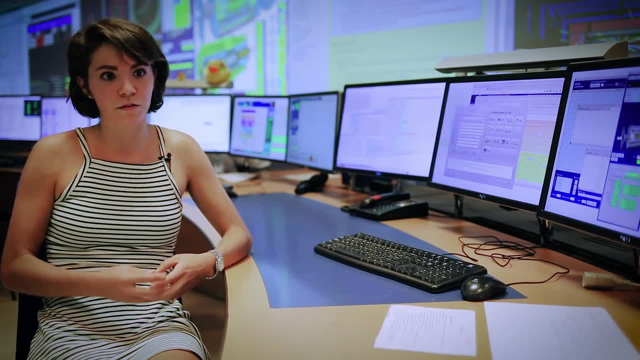 being surrounded by these really smart people Trying to answer the most fundamental questions in the universe.